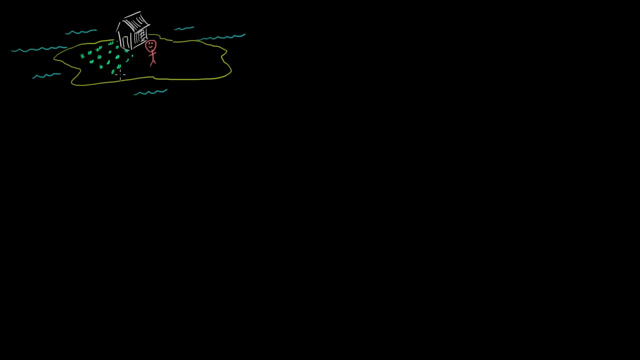 But he wants to think a little bit more formally about his economy And he starts setting up some institutions that start to resemble things that we would see in more complex economies. So what he decides to do is he decides to set up a firm. So let me put the firm right over here. 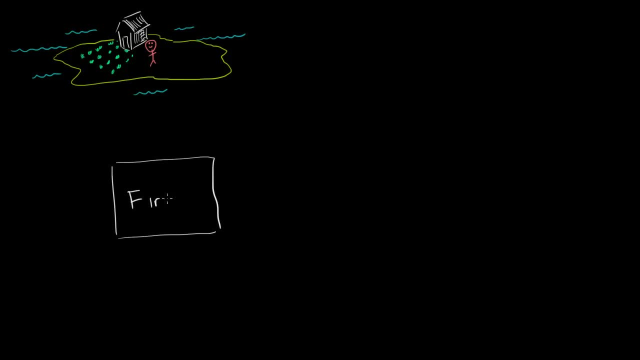 He decides to create a legal entity called some firm over here, some corporation, And he's sitting here. He's the household. He's a household of exactly one person. So this is him as a household. And he decides to give multiple factors of production to the firm. 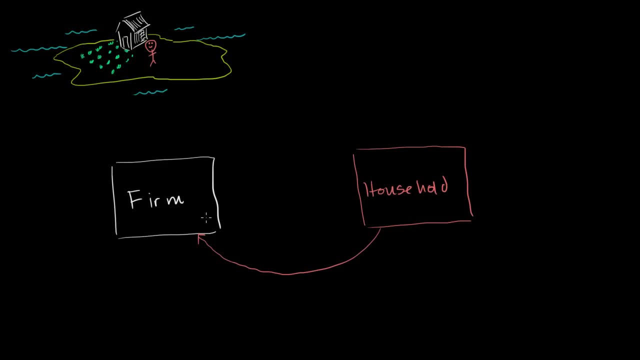 So he gives factors of production to the firm, So he essentially rents out his building, So he gives capital. He rents out the land to the firm, So he's giving land, And he also works for the firm, So he is giving labor. 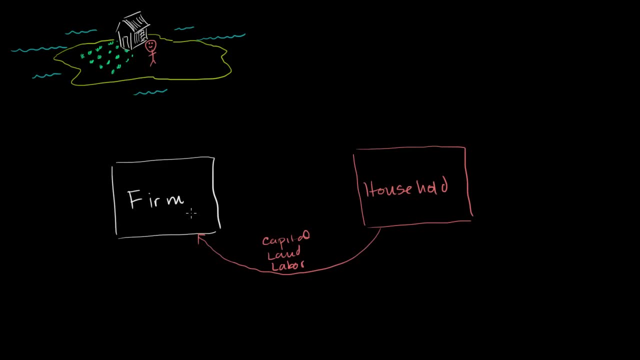 And he is the owner of the firm and he was the guy who thought of this entrepreneurial activity. So he's also giving the factor of production that's sometimes thrown in there as entrepreneurship Entrepreneurship. I'll just abbreviate it just like that. 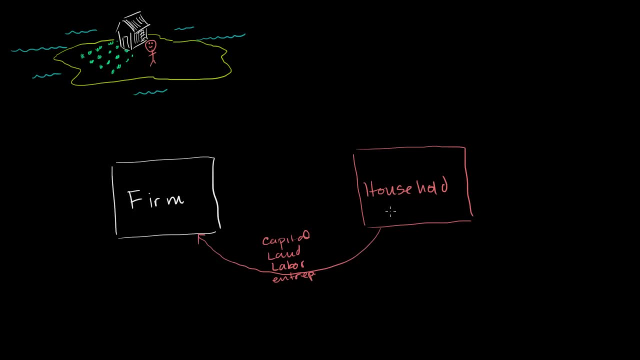 And in return the firm will essentially pay rents for these factors of production. So the firm will pay him money In exchange for being allowed to use all of these things. So for the rent on the capital, on the building itself, so for the building. 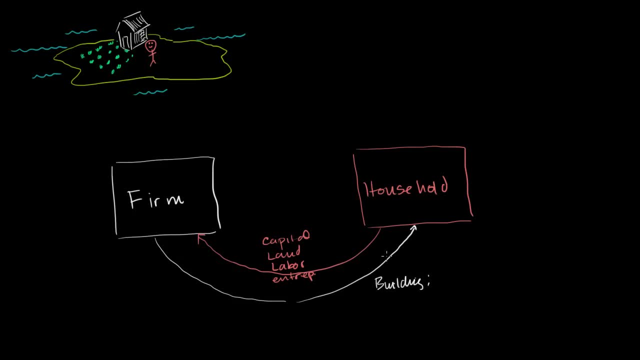 and we'll talk about. let's say, this is all in a given year For the building. the firm is going to pay him. the firm that he owns is going to pay him $1,000 per year. So this is the building rent. 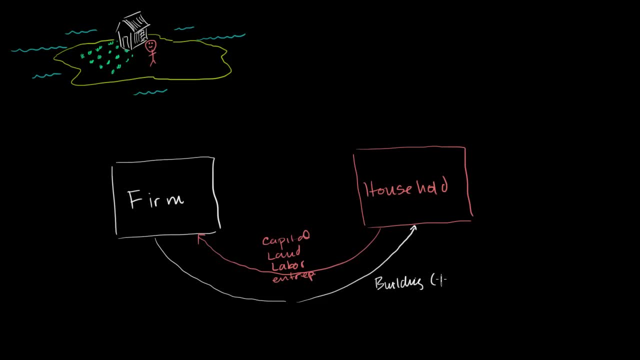 Let me make it clear that this is building rent or building lease. building rent Going to pay him $1,000.. For the land rent, he's also going to get paid another $1,000. And then for his wages, essentially the rent on his labor. so his wages- you could view that as rent on labor. 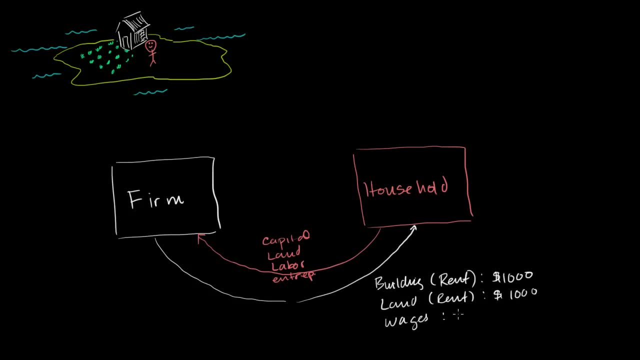 They're renting his energy and his time, His wages. he's also going to get $1,000 per year. Did I say $1,000 per month? It should be $1,000 per year. So he's getting $1,000 a month in building rent. 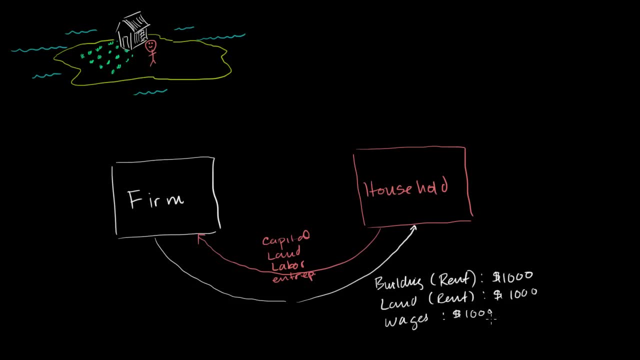 $1,000 a month in lease, $1,000 a month in land And $1,000 a month in wages, And he gets whatever profit comes from the firm because he is the owner of the firm And you could say that that's the compensation in exchange for his entrepreneurship. 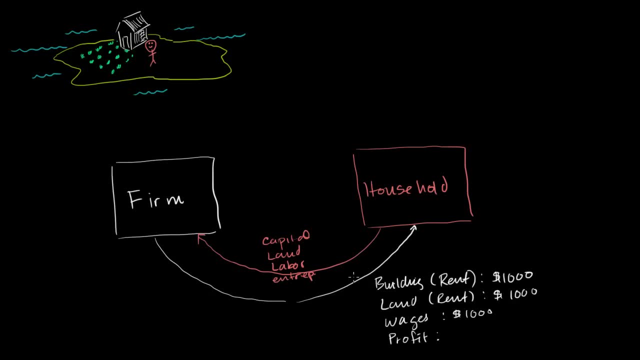 So looking at only this part or these two lines- the household- he is providing all of the factors of production for the firm so that the firm can produce useful things. So the firm can produce goods and services And it's good that the firm will produce good things. 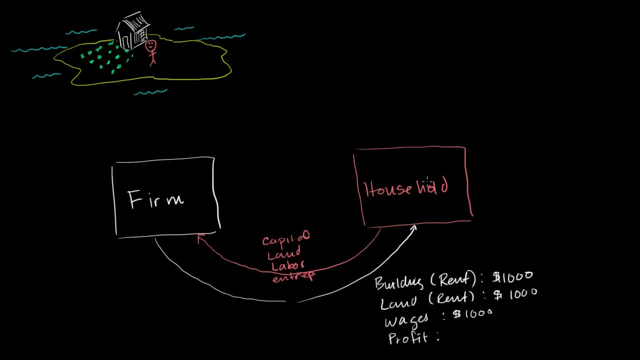 The firm can produce goods and services, because this household needs to survive, He needs a place to stay and he needs food to eat. And so let's say with the labor and this land, and so this guy's working at this farm. 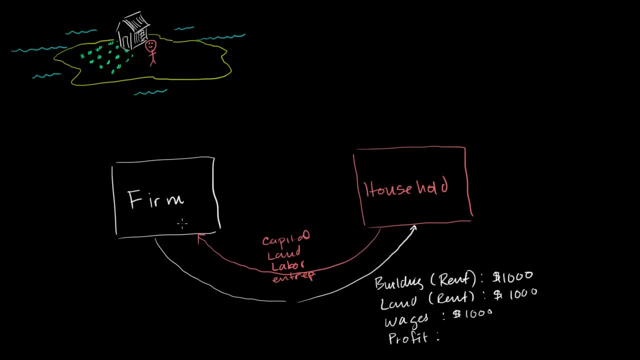 and it has this land and all of the rest, it's able to produce some food, And so it sells him goods and services. So it sells this household goods and services, and in particular it sells him food, and it also rents out the property. 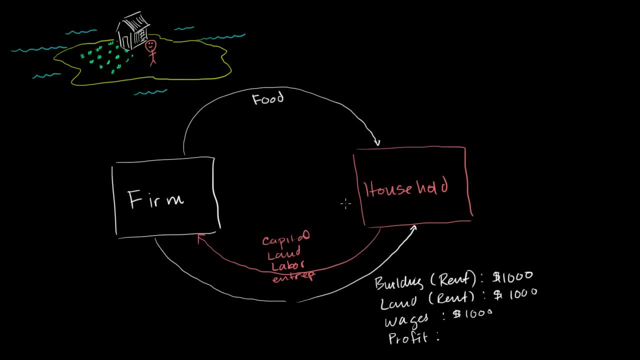 That's good, And I think you could see this is already getting kind of circular here. He's essentially renting out his own property, But this is a nice simple example. Obviously, once you expand beyond more than one person or more than one firm, things get complicated fast. 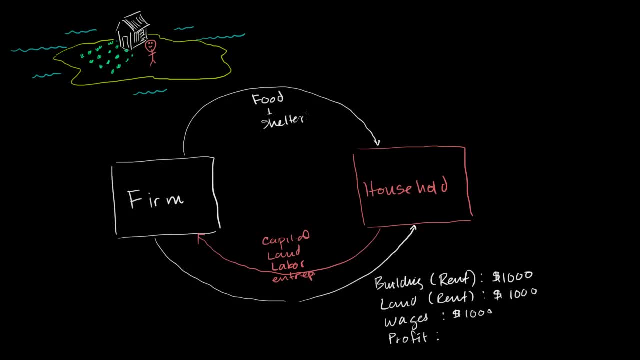 So he's getting food and shelter, And in exchange for the food and the shelter, he's going to pay the firm. In exchange for that, he's going to pay the firm, And so he is going to pay the firm. Let's just say that he decides there isn't much of a market right over here. 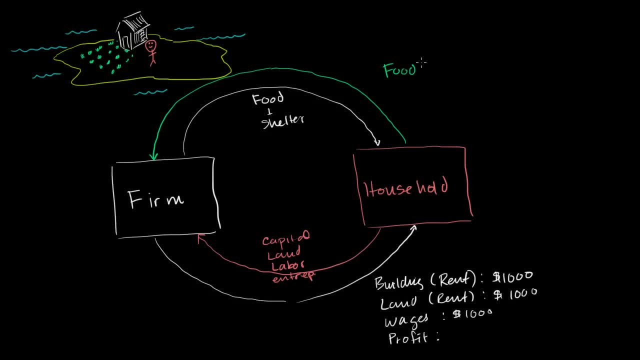 There isn't much of a market. but let's say, for the food he pays $2,300 a year. for the food And for the use of the building that the firm is renting, let's say he's paying $1,200, rent of $1,200. 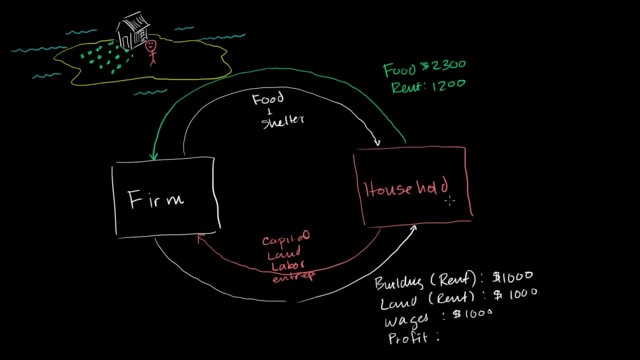 So a couple of ways to think about it. You could look at it from the household's point of view. What are his total expenditures? Well, total expenditures come out to what? $3,500.. So this is total expenditures for this household. 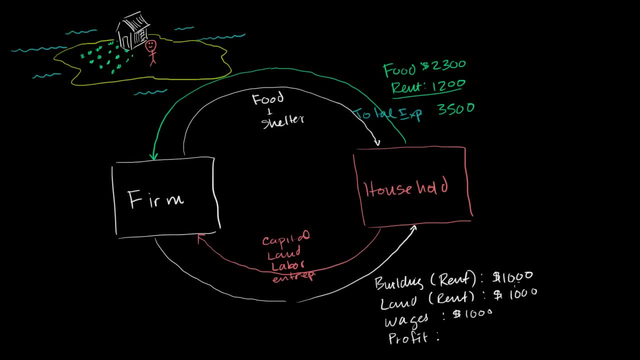 And what's his total income? Well, he gets $1,000 for the building, $1,000 for land, $1,000 for wages And he gets some profit from that firm. So we don't know what that profit is. 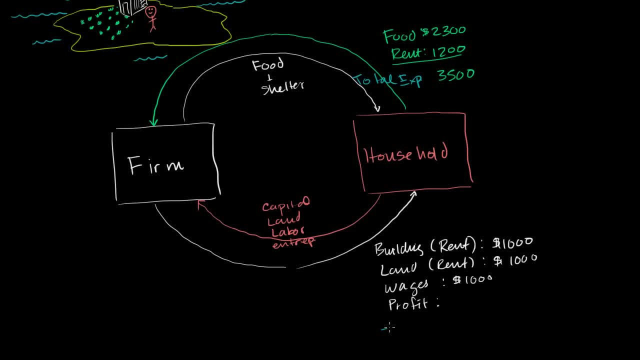 So why don't we hold off a little bit on his total income? So I'll just write it here: Total income. We don't quite know what that is yet, because we have to figure out how much profit he's getting from the firm. 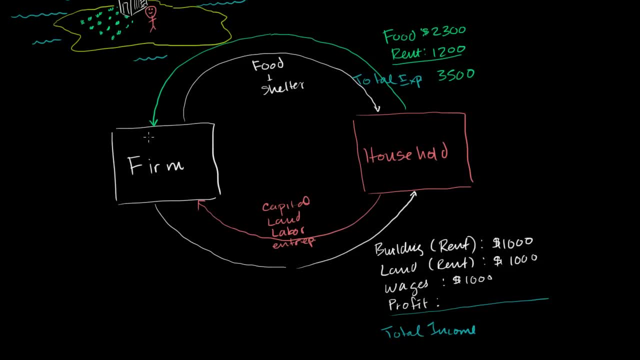 So let's look at the firm's point of view. What is the total revenue that they are getting For the firm? the total revenue? well, the firm is getting $2,300 for the food, $1,200 for the rent, getting total revenue of $3,500 per year. 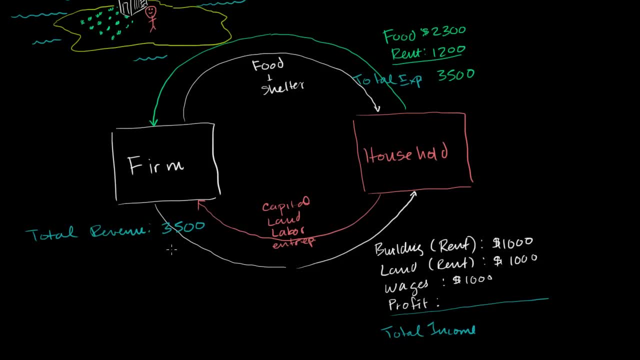 Everything here is on an annual basis. I have a feeling I said per month by accident, a few times. Everything here is on an annual basis, Getting $3,500 per year. And what are the firm's expenditures? Well, the firm has to, so this is expenses. 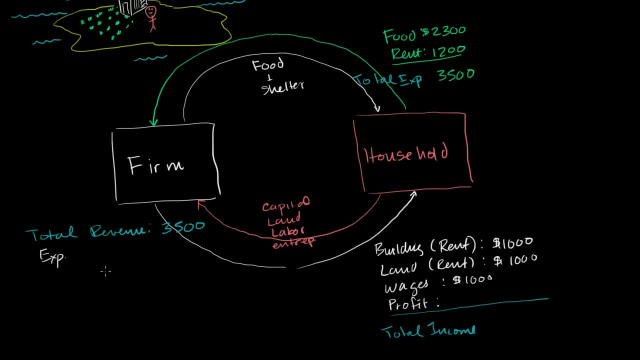 And here we're going to be thinking in terms of economic profit, because we're really just thinking about how much money is coming out of this firm, out of this business. So expenses, so for the building, the firm has to pay $1,000.. 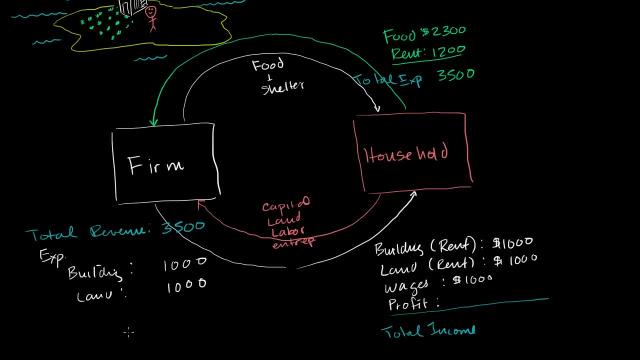 For the land, the firm has to pay $1,000.. And for the labor, the firm also has to pay $1,000. And so what's left over is the profit. We're assuming that there's no taxes over here. 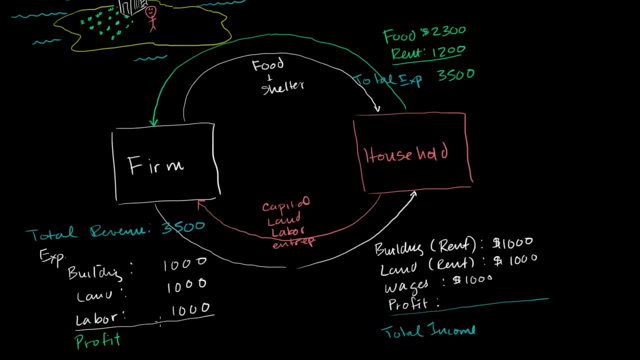 This is the profit for the owners. $3,500 minus $3,000 gives us a profit of $500.. And that's going to go to the owner of the firm, who happens to be this guy right over here. So the profit is $500. 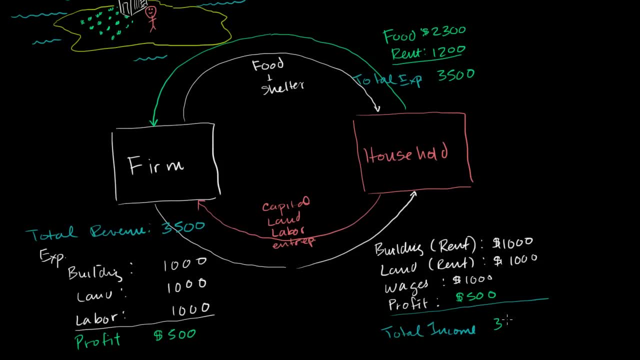 And so his total income is $3,500. And it's good that his income is at least $3,500, because that's how much he's spending it per month. Spending per month, Spending per month. Spending per month. And the reason why I did this is to kind of show you the circular flow of goods and services. 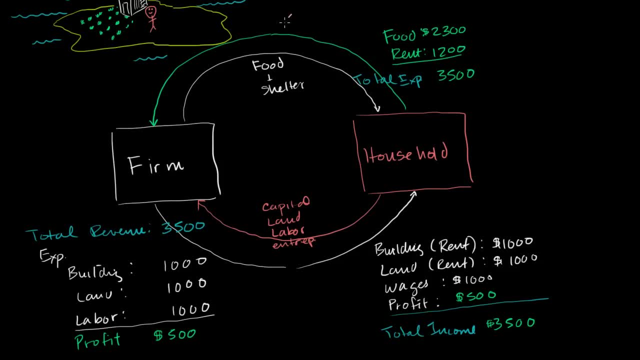 These are the goods and services up here. Let me show you. These are the goods and services. Goods and services. The firms provide the households goods and services. And then the households are providing the firms the factors of production. And sometimes you might say, well, aren't other firms also providing the factors of production? 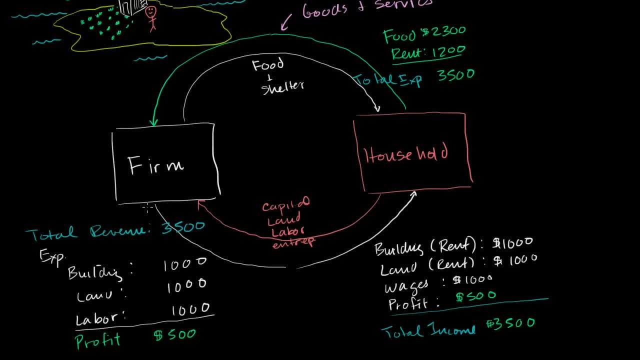 Yes, other firms could if there were other firms. But those firms, at the end of the day, are owned by someone. They are getting their factors of production By some, By some household, Or they are owned by some household. So you can view it as, at the end of the day, the households are really giving the firms the factors of production. 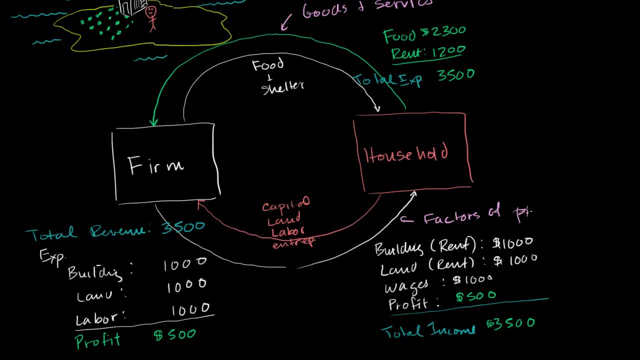 Factors of production And in exchange for the factors of production, the households. in exchange for giving these things, the firms give the households income, essentially rents on the different factors of production that are being given to the firm for the most part And over here, in exchange for the goods and services. 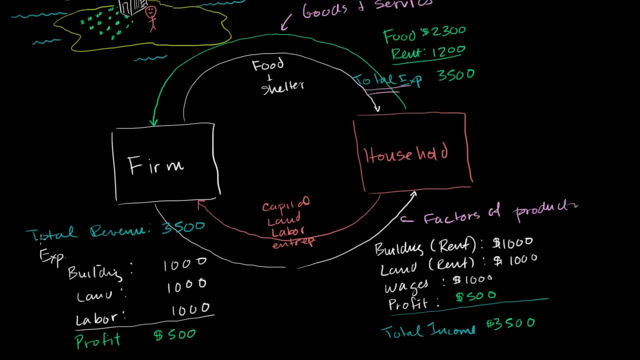 the households are making expenditures that can also be considered revenue of the firm. Now, if you were an economist that were to observe this, and I guess if we were to focus on this island, maybe he would also have to be the island economist. 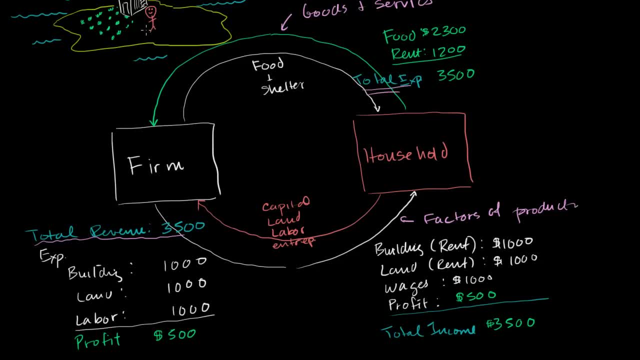 and you would say: how would you measure the total value of the production of my country here? Maybe we could call it the gross domestic product? How would we measure it? Would you count just the total expenditures or would you count the total expenditures? 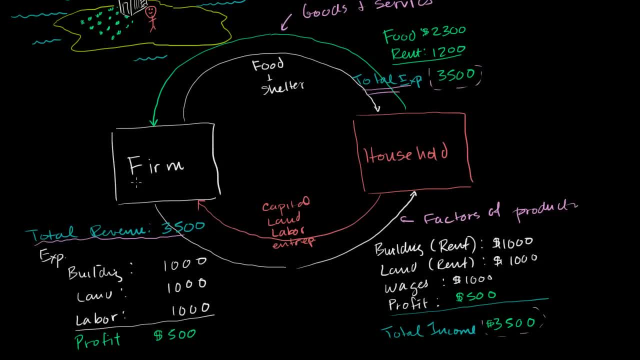 And the total income, Or would you even count that and the revenue? Well, if you counted all of that, you would be essentially triple counting. If you counted the total revenue, the total expenditures and the total income, they're all that $3,500, you would be triple counting. 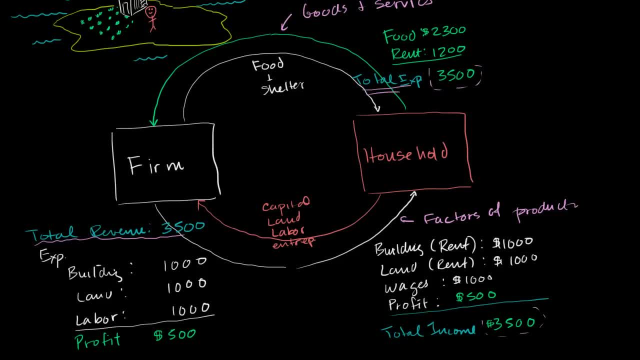 So what you could do? you could just measure only one of these things. You could say: your GDP, your gross domestic product, is the total expenditures by the households. So it would be the $3,500.. You could say it is the total income. 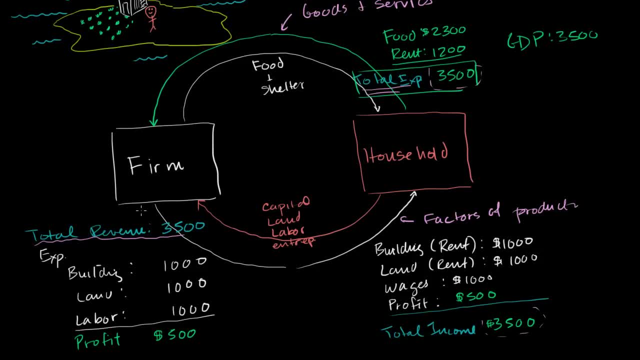 by the households. So that would also be $3,500.. And the total revenue really is the same thing as the total expenditures. So the whole point of this video- and this is obviously a very artificial case where we're dealing with an island with only one person-